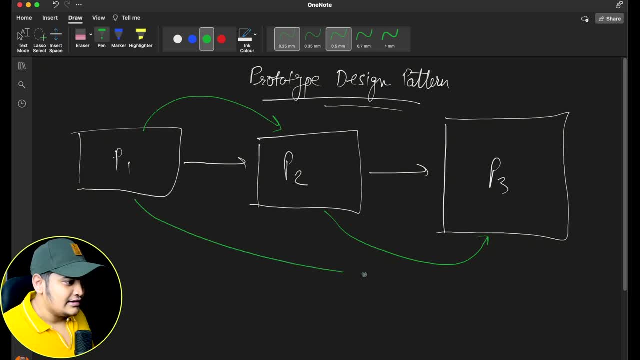 to have the another prototype, or I can do little tweaking on the this prototype itself and can create the another objects as well, or another prototype as well. So you can see that, based on some base structure, you will be creating the different objects. So that's. 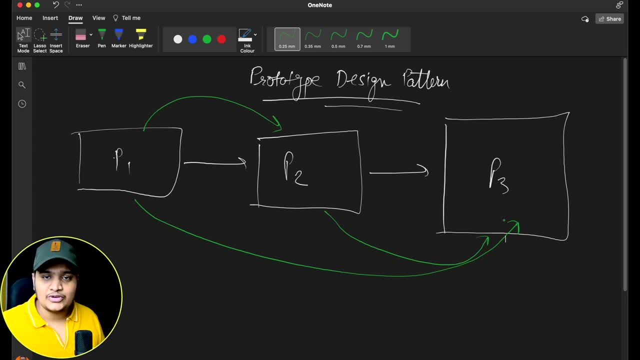 where prototype design pattern comes into picture. So suppose, if you have lots of objects to be created and all those objects are very heavy while creation process, So what you can do is You can create the prototype pattern out of it and you can create the clone of that particular 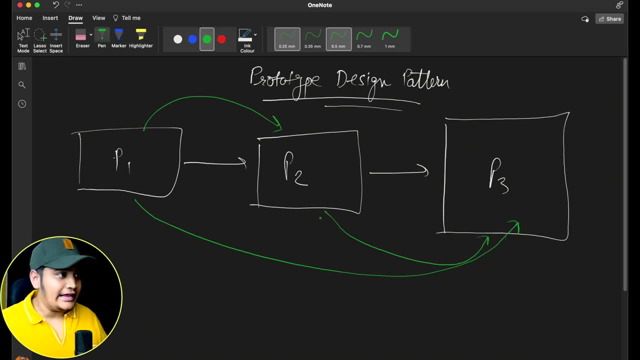 prototype and you can do some modifications. Okay, So you can see that we are not doing any rocket science here. whatever the prototype it was earlier we did some tweaking on it and then we created the different prototype. So for our objects as well, if I have objects. 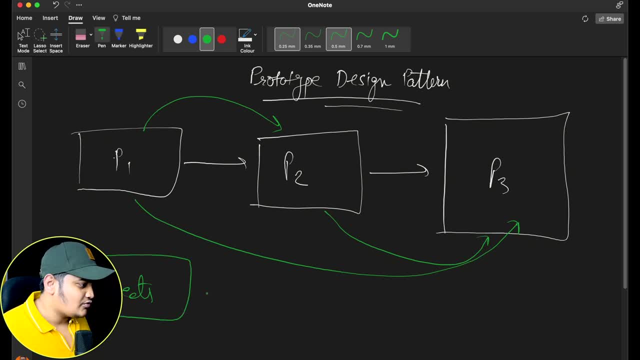 created, okay, And for that objects, what I can do is I can do some tweaking on it and I can create the objects. So when I have to do the tweaking, what I will do is I will clone this entire object, Okay, And then I will create the prototype pattern out of it. 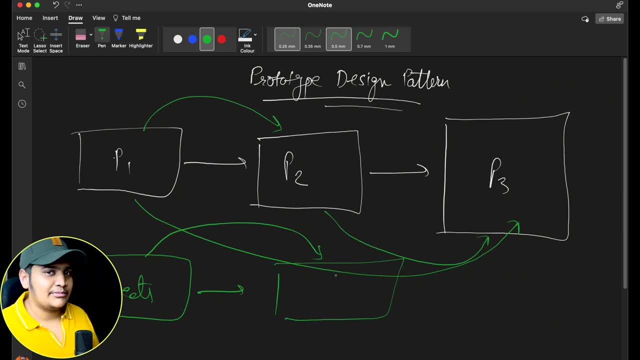 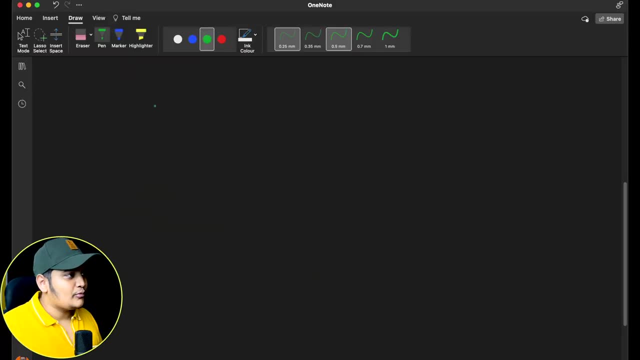 I can create each object, do some tweaking on it and then I can use that particular object. So that's the idea behind the prototype design pattern. Let's understand more on it. So let's understand with one example here. So what we can say here is suppose you've 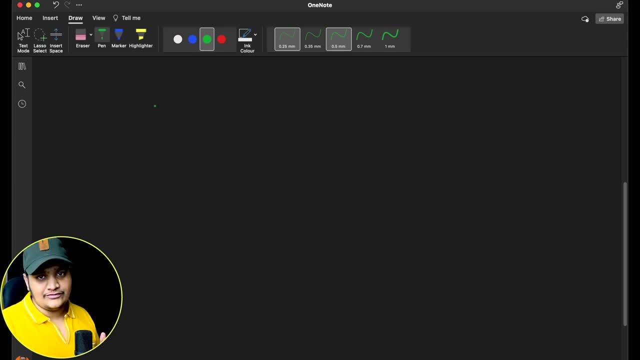 want to create two wheelers and four wheelers. okay, The objects of two wheelers and four wheelers. So how you will create the object of those things? So suppose, if you have the base thing, so the base thing offered- two wheeler and four wheeler would be vehicle. 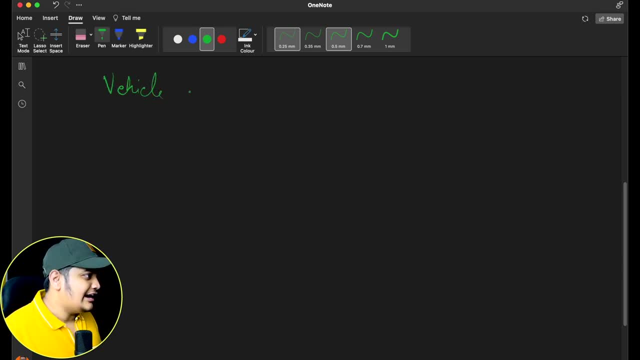 right. So you would be creating a vehicle and with that vehicle, either you can create a two wheeler or you can create a four wheeler. Okay, And if you are using the two wheeler for your object, you can also create a four wheeler. 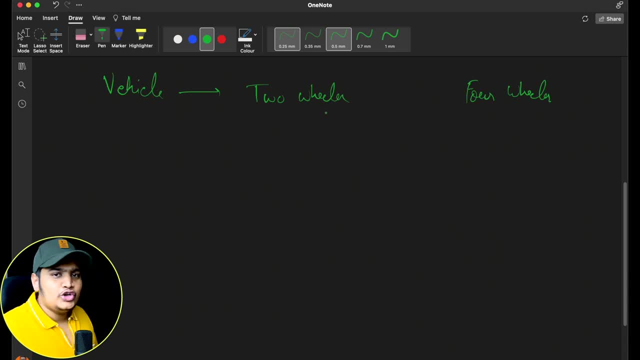 you can create a four-wheeler or a car, whatever you want to say, because in two-wheelers also you can create a bike or motorbike or a scooter. in four-wheelers you can create a pickup truck, you can create the car- so many stuffs okay. so that's why we are going with a generic form. now. you can. 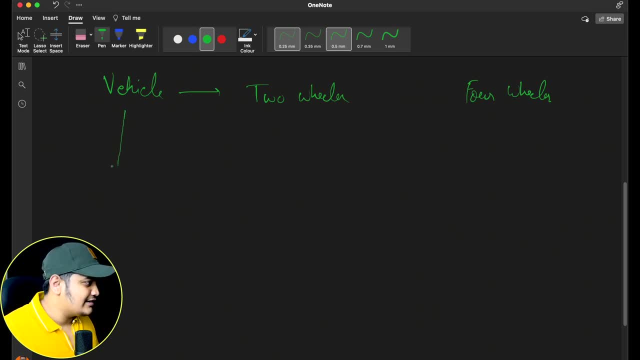 see that what vehicle would have? okay, so vehicle would have basic things. so vehicle would have engine, what model, it is okay. the price of the vehicle and lot more. okay, so you can see that this is your base vehicle. okay, this is your base vehicle. now, based on this base vehicle, you can. 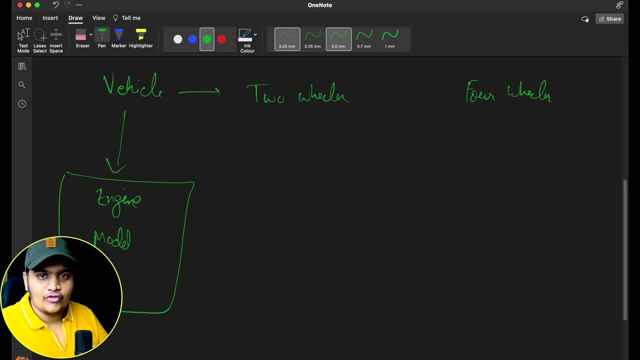 either create what type of that vehicle is. either it's a two-wheeler or four-wheeler, okay. and to have everything added here as a vehicle, it's a complex task, right? because creating vehicle itself is a complex thing. so what we are trying to do is, rather than creating the object of a vehicle or a 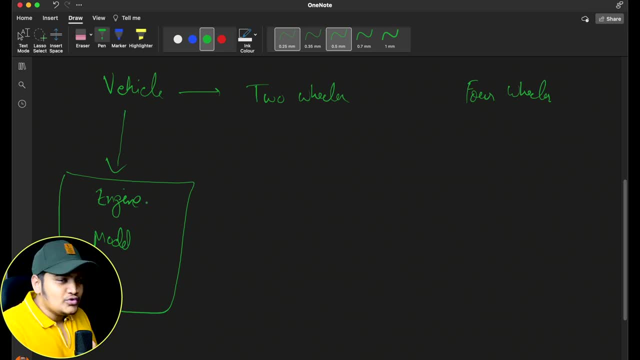 two-wheeler or four-wheeler. every time, what we can do is we can use the already existing objects and what we will do is we will clone that particular object and we will do the picking on it. so what i want to do is, whenever i want to create the two-wheeler, what i can do is i can define: okay, it has to be a. 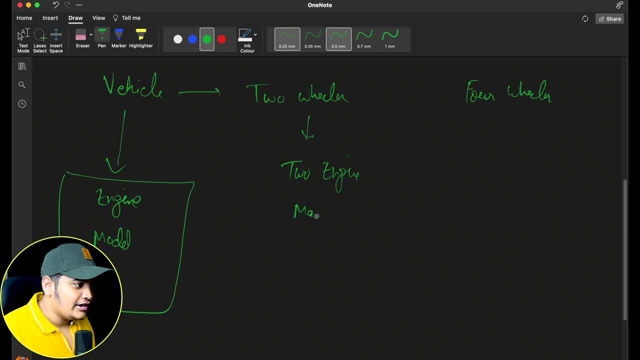 two-wheeler engine, it should have a particular model for it. it should have a price for it. okay, i can add some more parameters as well here. suppose, is this two-wheeler electric or not? that also i can define, okay, and so you can see that this is something that is the deciding. 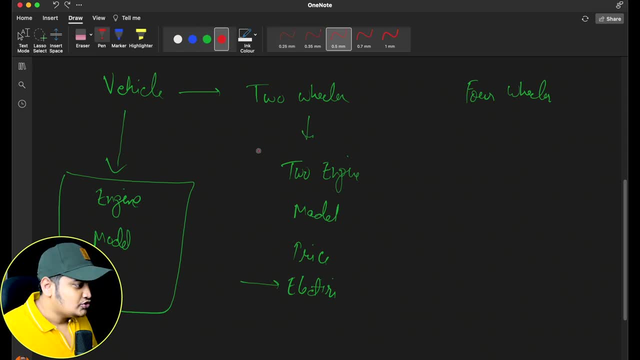 factor or a change factor based on the default vehicle. so you can see that with this particular change, you can see that you had created the object, but most of the things were similar, most of the things that you copied from the vehicle object itself. so what you did? you copied the object here. 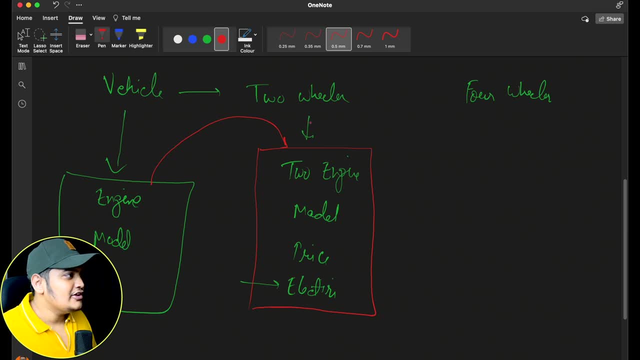 okay. and then you added some of the properties. similarly, you can do the same thing over here as well. so in the four wheeler as well, you can add the engine, you can add the model of that engine, model of the car, the price of the car- is it going to be petrol car? is it going to be? 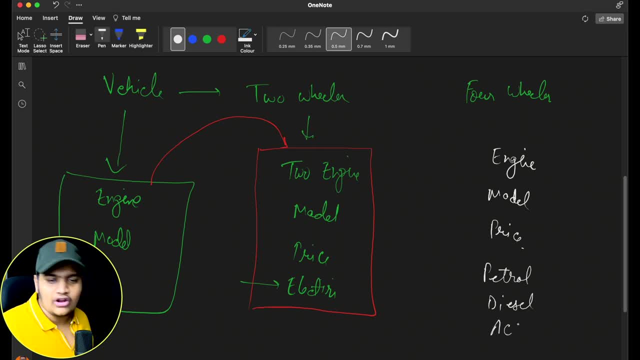 diesel car. whatever it is, is it going to be having the air conditioner or not? whatever, there are different parameters to it. you can add the different parameters. so here also you can see that few of the things you are taking from the vehicle object itself. you will be cloning this. 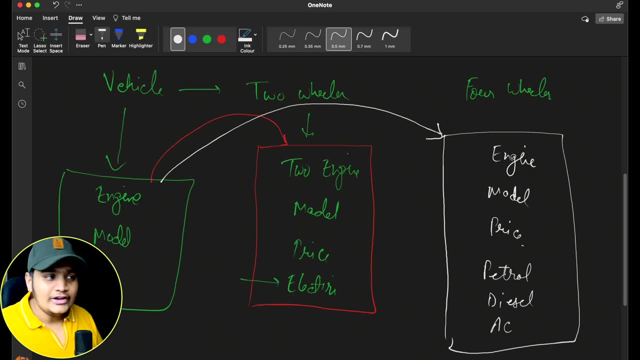 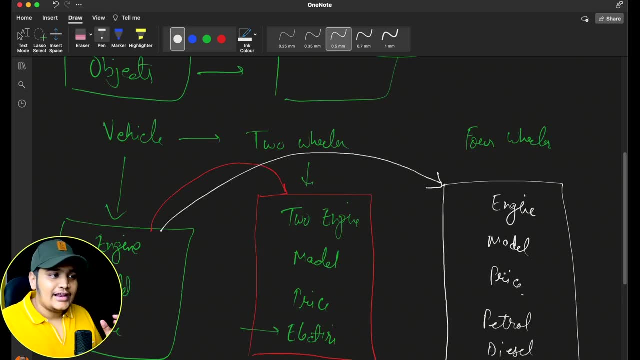 object and you can add the different parameters to it, so you can see that you are using the base object, that is, the vehicle object. on top of that you are doing some modifications. so one more thing we can do over here is we can have the registry of the prototype objects that we can create. so 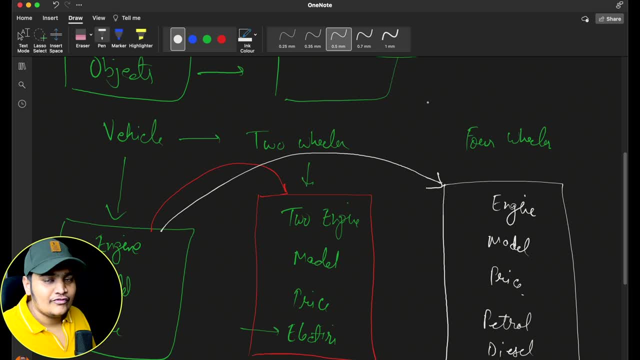 rather than cloning this object every time for a two-wheeler or four-wheeler, what we can do is: i already know what i want to have in a two-wheeler and i already know what i want to have in a four-wheeler. okay, so those objects as a base objects. okay, these two objects as a base object. 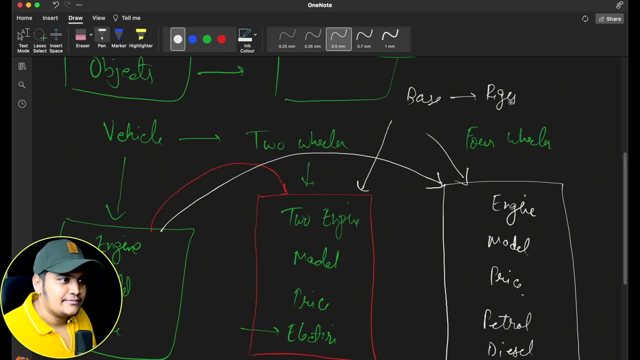 i can store somewhere right and that i can store in the registry. don't mind my spelling and handwriting, it's really bad, okay. so just understand that this image and this image, okay, that is the two-wheeler object and the four-wheeler object. so 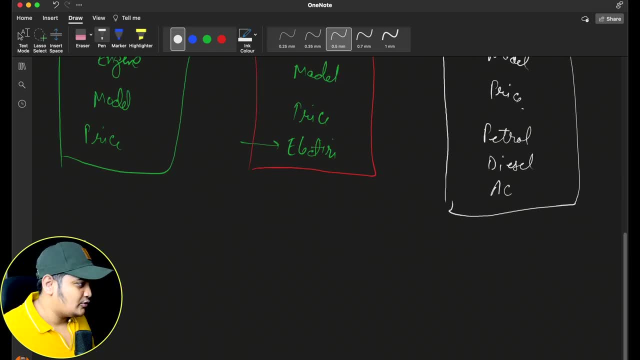 i can store in the registry. okay, so suppose i can create a vehicle registry and in this vehicle registry i can store that two-wheeler object and a four-wheeler object, and i can store each and everything in a hash map, and here i can give a key as well. this is going to be two, this is going to. 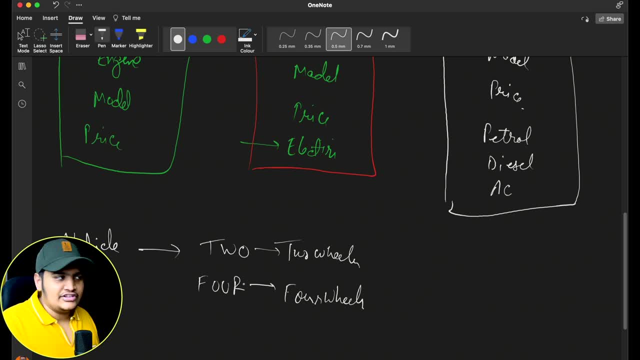 be four. so now you can see that i have the base object stored in one registry. okay, this is going to be my registry now. whenever i want to create a two-wheeler, okay, what i will do is i will clone this object. i will clone this object of a two-wheeler and 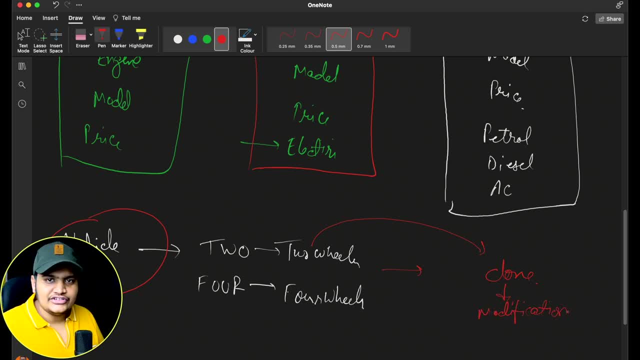 whatever the modifications i want to do, i can do those modifications and i can have the object of a two-wheeler. similar thing: when i want to have the four-wheeler object, i will just get this object, clone it and i can do the modifications and i can have the four-wheeler object. so you can see that. 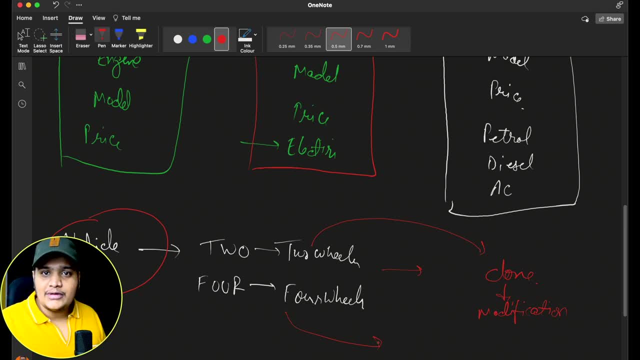 every time. i do not have to create the entire object by myself. there is an already object available in the registry. i can use that object and i can do the modifications on it and i can use that object directly. so you can see that there will be a lot of time saved while creating. 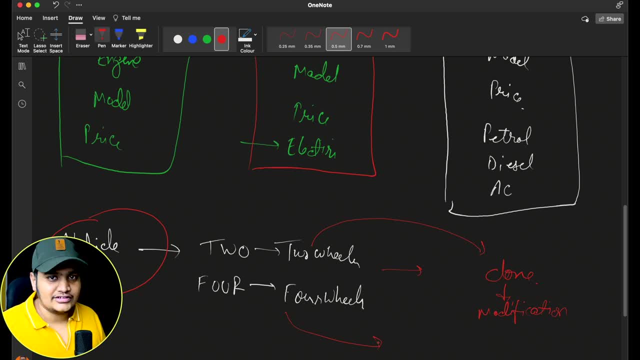 the objects, because these objects will be very heavy while creation processes. okay. so that's why we are using the prototype pattern. if the object creation is heavy, at that time only we should go with the prototype design pattern, create the prototype of it and clone that particular prototype and use it. okay, so you can see that the cloning part is really important here. so this is. 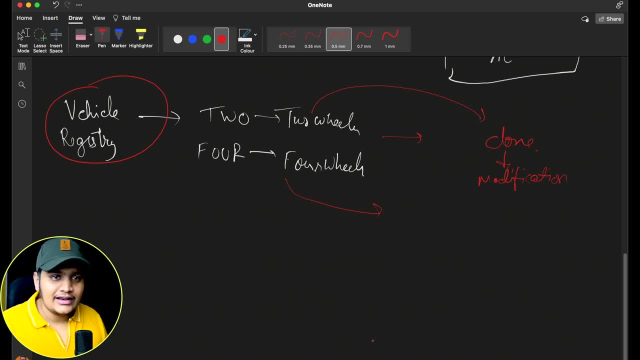 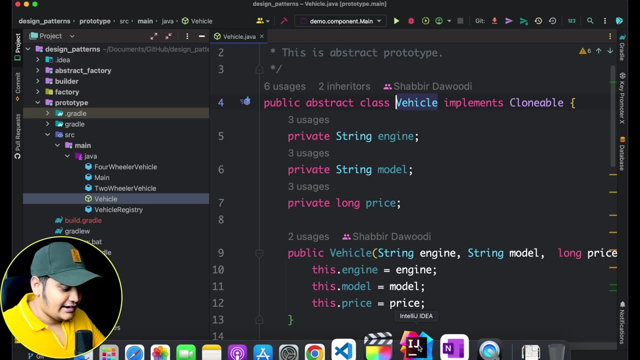 just the high level explanation that i have given you. let's understand by code as well, like what we mean by vehicle registry, what we mean by cloning and everything. okay, so let me just go to the intellij idea here, and here you can see that i have the prototype project available. okay, 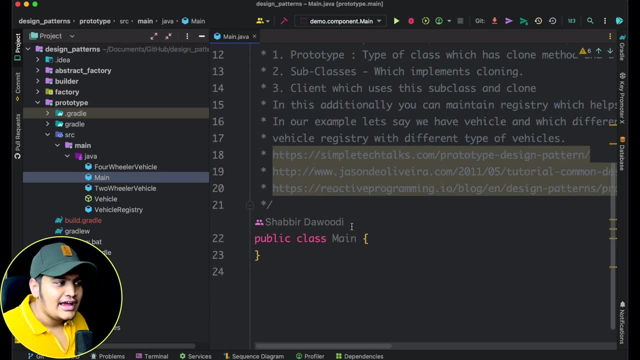 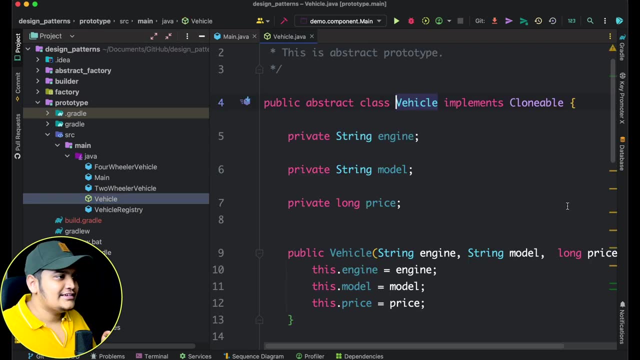 in this prototype. you can see that i have given the entire explanation here and i also added the reference from where i have took this example. okay, so you can refer this as well. i will share all the codes with you. so here you can see that i have created a base vehicle here and you can see that. 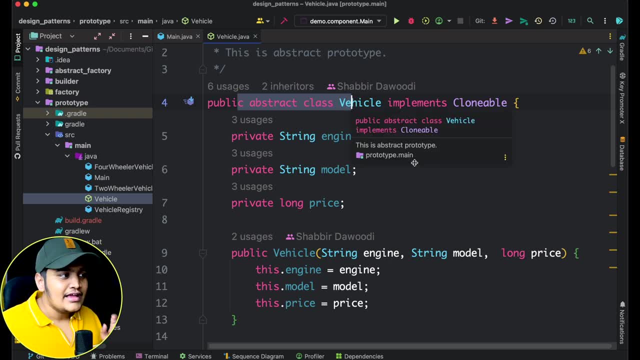 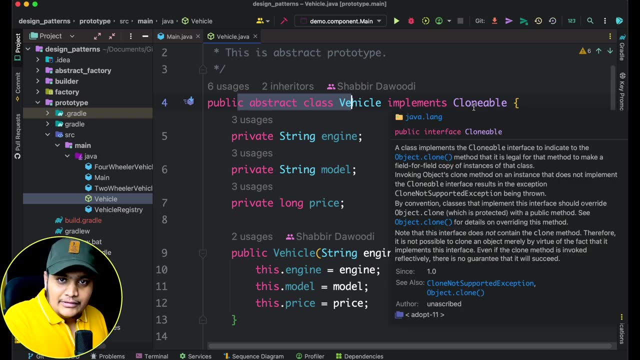 this is the abstract class vehicle. this is the base class that we understood earlier, and you can see that this is implementing clonable interface. so this part is really important, like whatever the code you are keeping for a client to use that has to have the capability to clone the particular 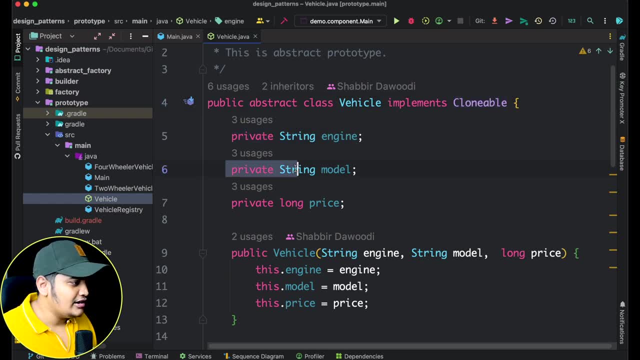 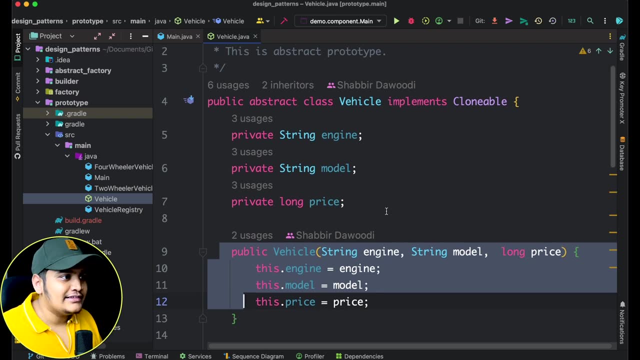 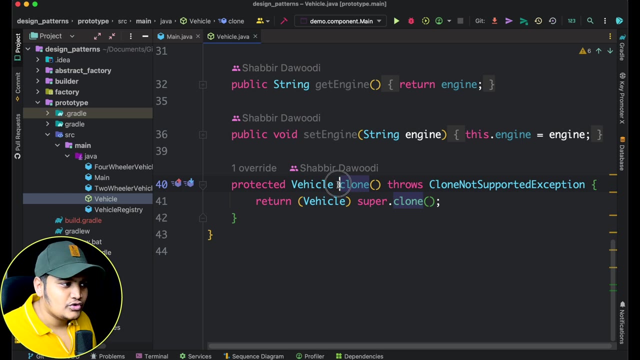 object. so you can see, within this vehicle we have engine model, price and a constructor which will initiate the object of a vehicle. simple thing, okay, one more thing: you can see that as we have implemented the clonable interface, we also have the clone method here, and you can see that what? 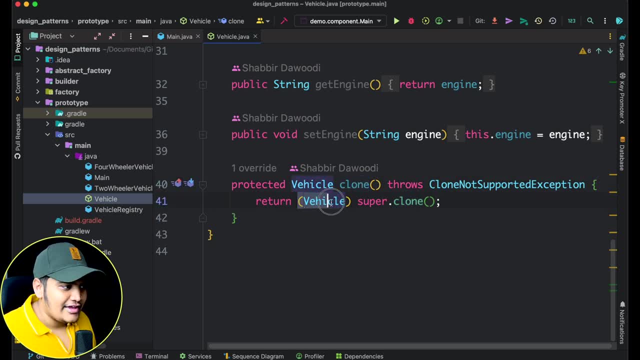 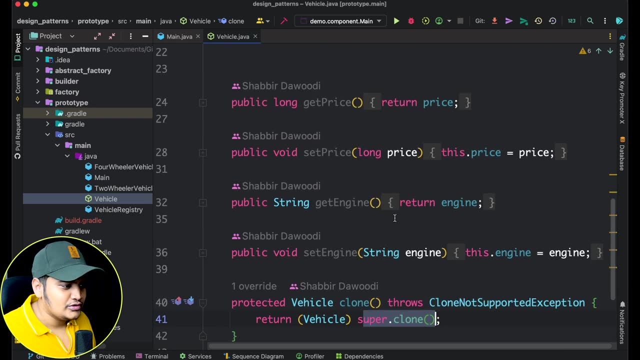 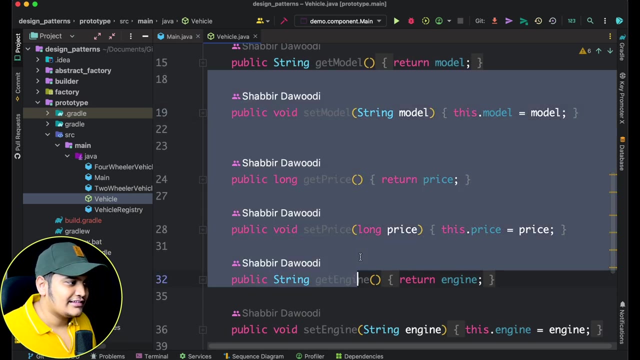 this clone method is doing. this clone method is returning the vehicle object by doing the clone. and if we have created the clonable interface, we can do the clone operation here and it will clone the object, convert to vehicle and it will return it. and this all different methods. you can see these. 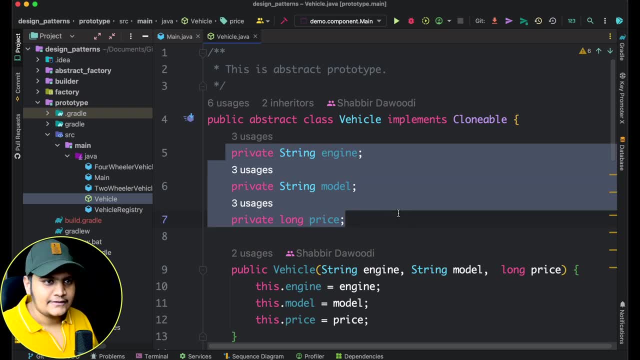 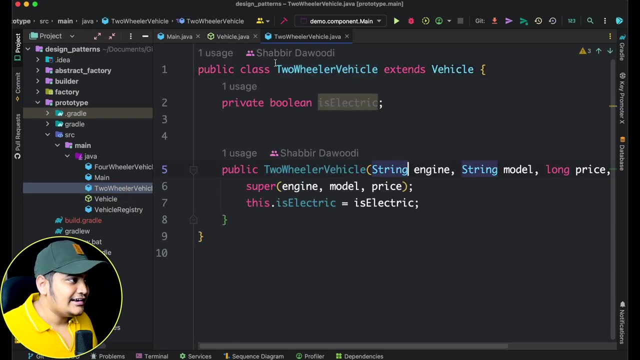 are thus the getters and setters for these three values. simple thing now: your base vehicle class is ready. now let's go to two-wheeler vehicle and a four-wheeler vehicle. so if i go to two-wheeler vehicle, you can see that this two-wheeler vehicle is extending the vehicle itself. okay, and it has. 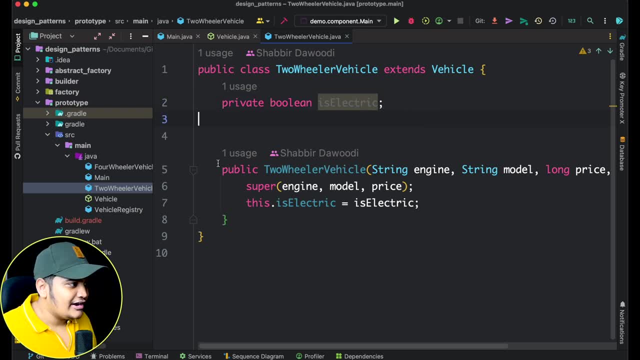 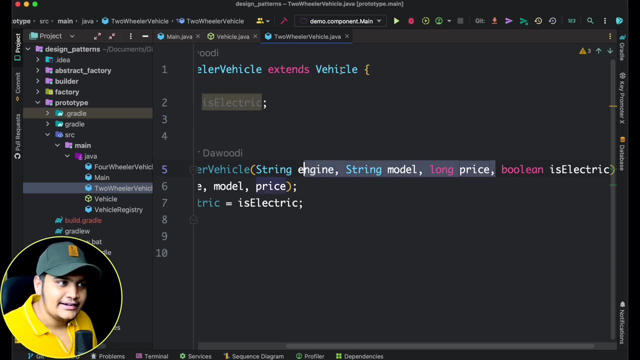 one extra property, that is it electric or not? now you can see that whenever i am creating the object of it, what i'm taking is: i'm taking the engine model price. these three are part of the vehicle itself and i'm taking the is electric as well. so i'm calling the super and i'm assigning. 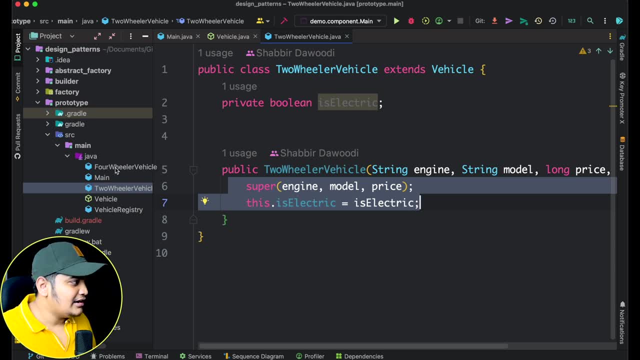 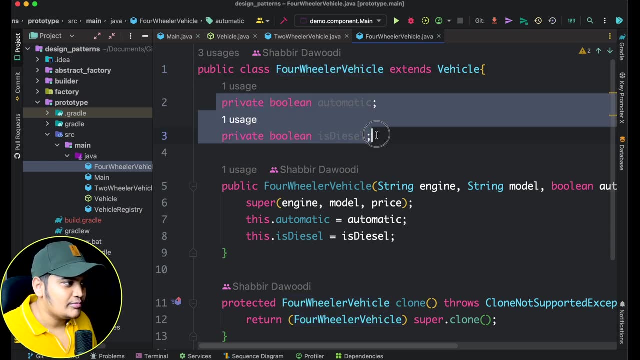 these electric as well. simple implementation of the two-wheeler. similarly, if i go to the four-wheeler vehicle, this is also very simple. four-wheeler vehicle is extending the vehicle class. it has couple of more properties and it has a constructor to initialize the object and 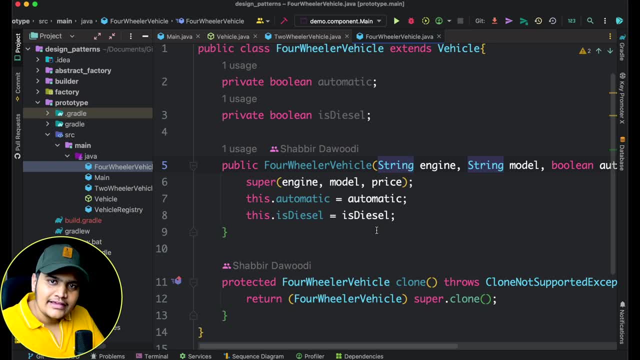 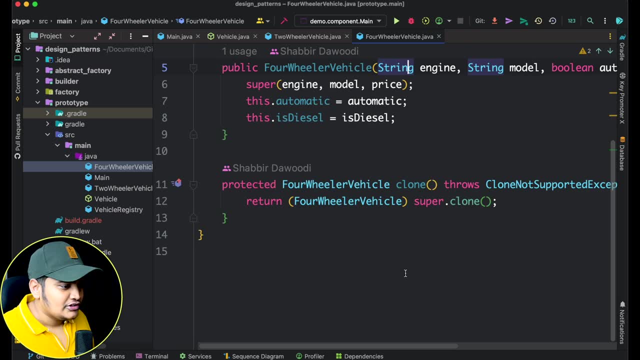 a clone method as well. so whatever classes are extending your base class, all those classes should also support the clone method. okay, that's the main thing over here. so here also you can see that it is supporting the clone method and it is cloning the object and it is converting to four-wheeler. 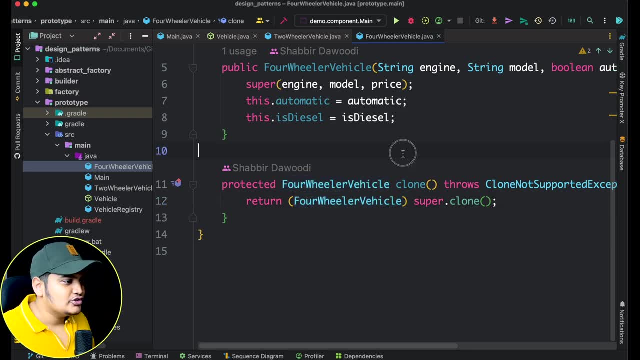 vehicle here. okay, similarly, it has to be in the two-wheeler vehicle as well. so you can see that vehicle, two-wheeler vehicle and four-wheeler vehicle. all should have the clone methods. so now all your base classes are supporting clone methods. so whenever i want to get a particular object, I 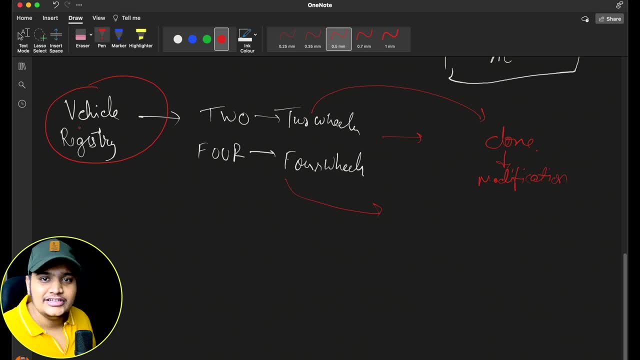 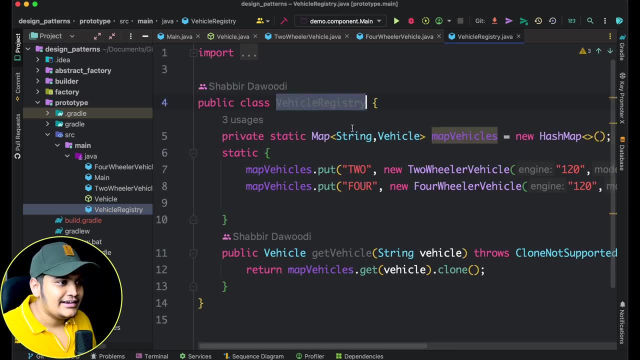 like the classes only we created. but now you can see that I have also mentioned the registry as well. so here you can see that we have created the vehicle registry as well. so this vehicle registry, you can see, that is nothing but a hash map of string and vehicle. okay, so you can see. 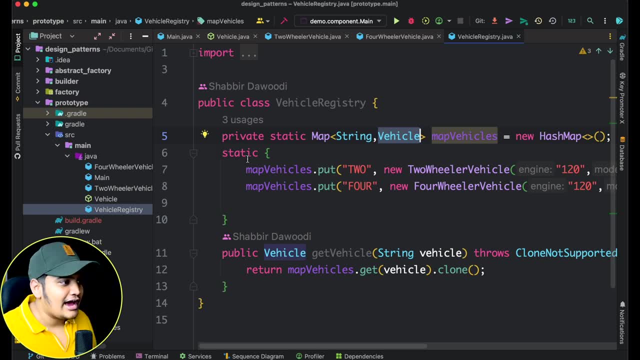 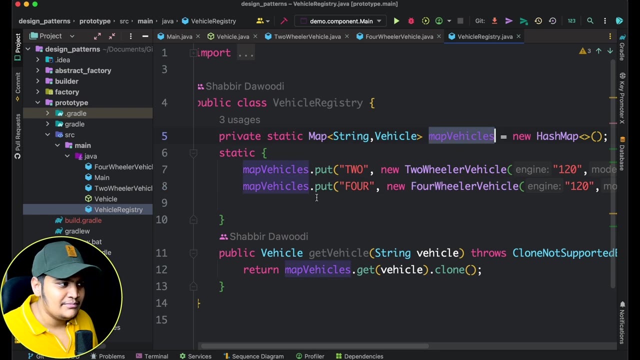 that, within the starting of the application itself, what I'm doing is I am creating the prototypes and storing in my registry. simple. so I am creating the prototype of two-wheeler vehicle and a four-wheeler object and I am storing all those objects in my registry. that is the map vehicles and with the 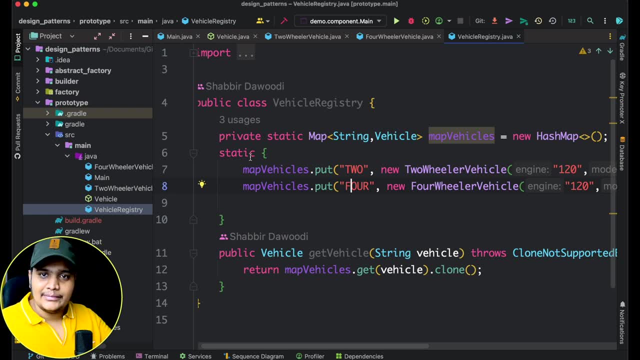 key is 2 and the key for the four-wheeler is 4.. so you can see that whenever my application starts, I have the prototype objects ready. now, whenever anyone wants to use those objects, they can get using one of the methods that we provide. so here you can see that we are providing get vehicle. 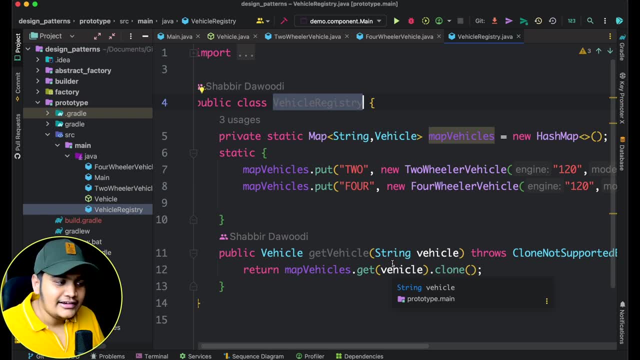 method from the vehicle registry. so whoever wants a particular object, they can get directly by the value that they pass. so suppose they want a object of two-wheeler, they can pass two year as a string value and what we will do is we will get a. 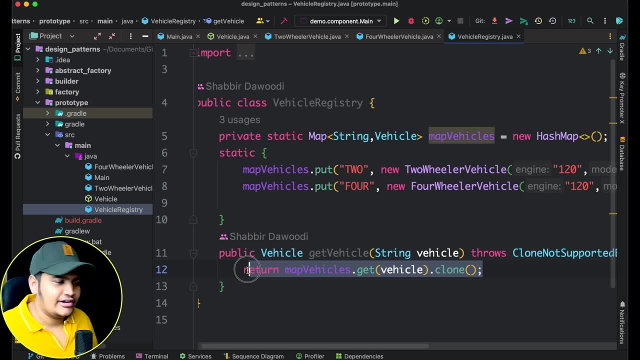 particular two-wheeler object from the hash map and we will clone it and we will return it. simple, so you can see that from the registry itself we will provide the client to get a particular prototype object, that is, the clone object of a prototype we have already stored. similarly, if 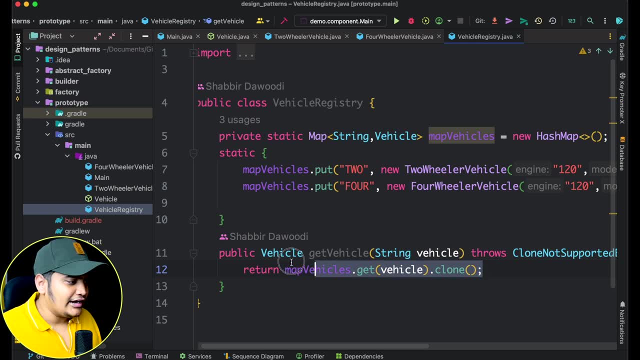 they want the object of four-wheeler, they can pass four and it will clone it and it will return the particular object. so you can see that the objects will be always new created. it will be a clone of the object that is already created. whatever the modifications needs to be done, that modifications